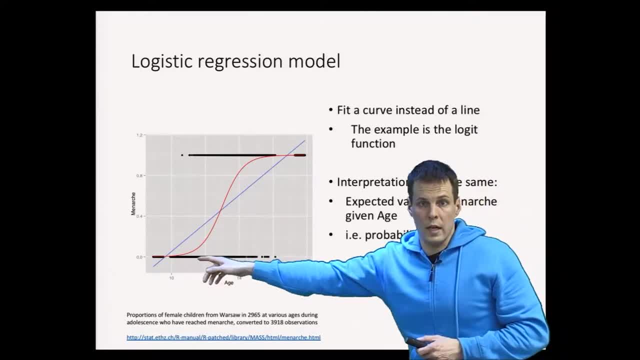 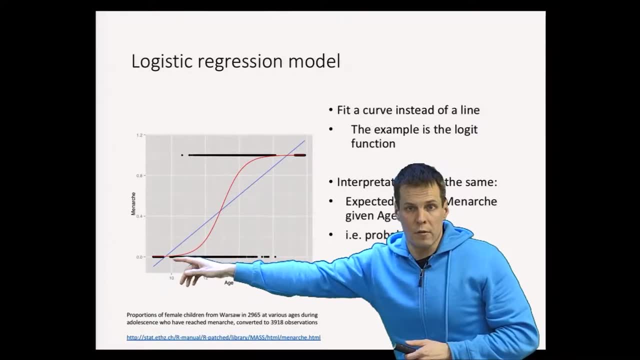 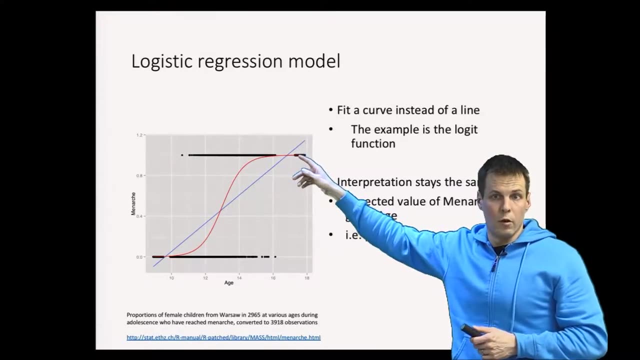 the logistic curve. So we can see here that when the girl's age is close to 10, which is the minimum in the sample are, the predictive probability of menarche is about zero, and when the girl is 18, which is about the maximum of the sample, the predictive probability of menarche is about one. 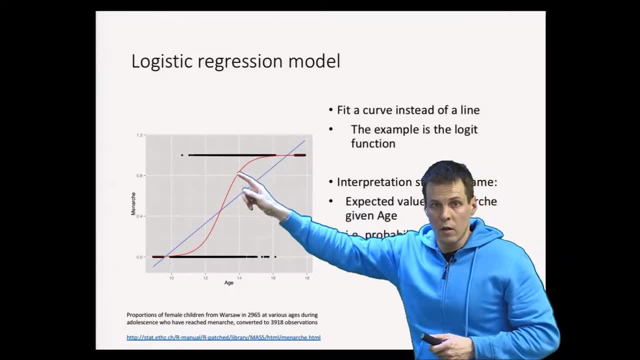 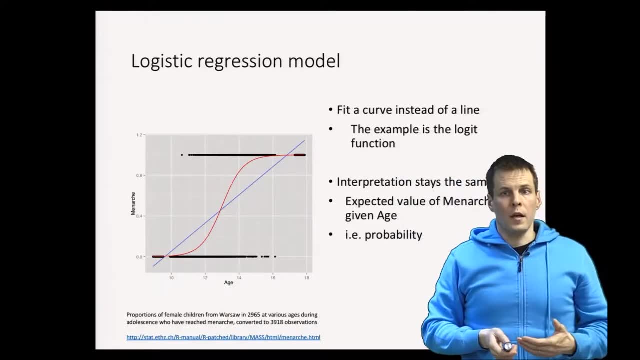 And we want to estimate this logistic curve, how it goes and it tells us the relationship between age and menarche. We apply the probability calculations to values that are ones and zeros, That's the dependenteses variable, and to do that we use the Bernoulli distribution, The idea of a Bernoulli distribution. 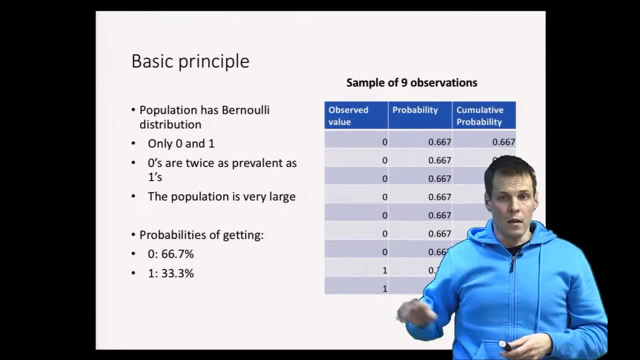 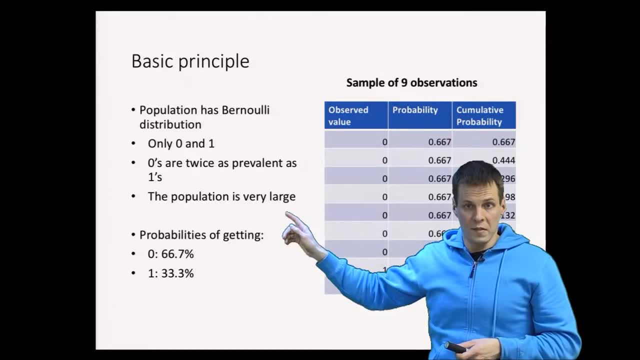 is that we only have ones and zeros and in this example the zeros are twice as prevalent as ones and the population is always very large in maximum likelihood estimation, because when we take a sample of one, one zero or one one away from the population, the ratio of ones or zeros should stay. 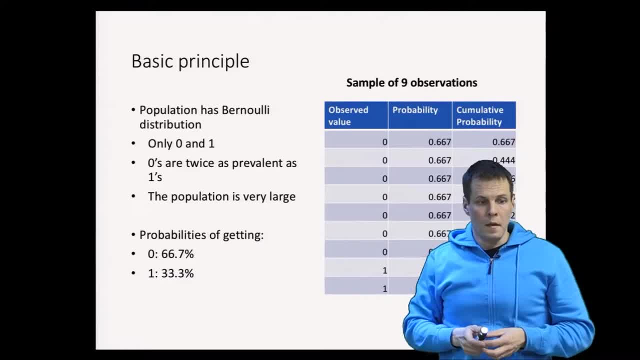 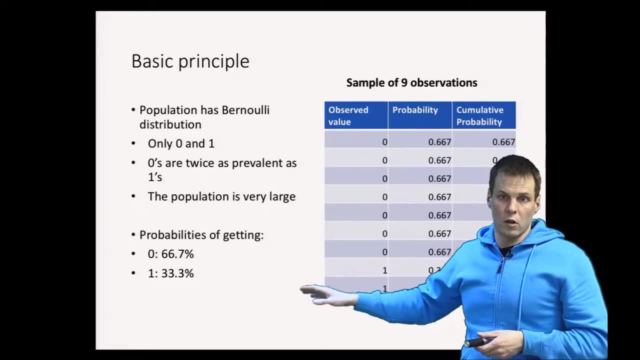 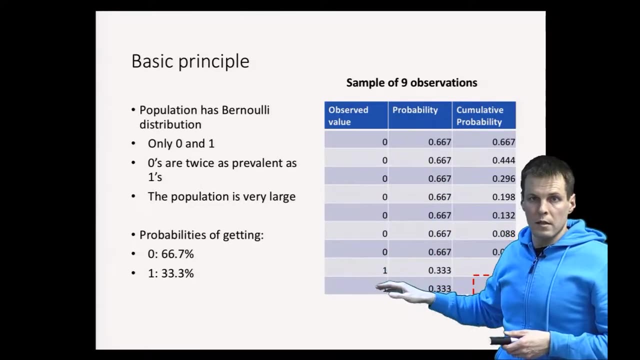 the same even if we take a sample away from the police. The probability of getting zero is 67% from this sample and probability of getting one is 33%. So when we have this set of observed values that are sample, we have seven zeros and two ones. they happen to be in this order by random. 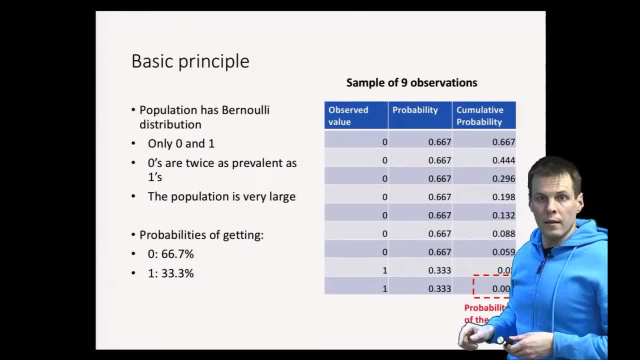 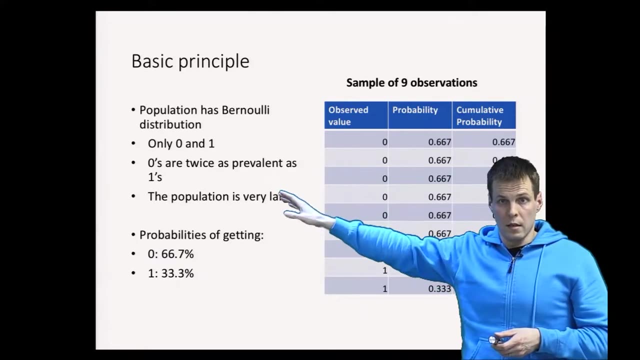 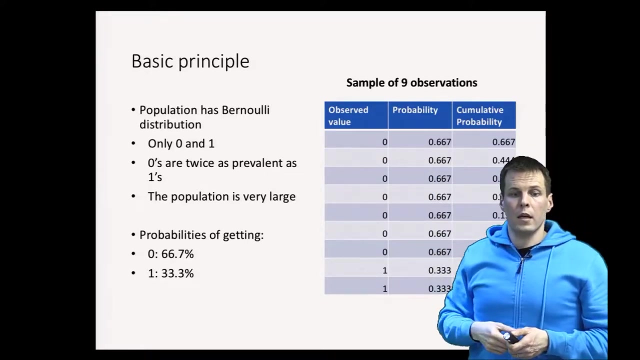 it doesn't have any significance or any meaning. and we calculate the probabilities, then we calculate the total probability by multiplying all these individual probabilities together. So when we know what the population is, then we know the probabilities of getting particular values from that population In maximun likelihood estimation. 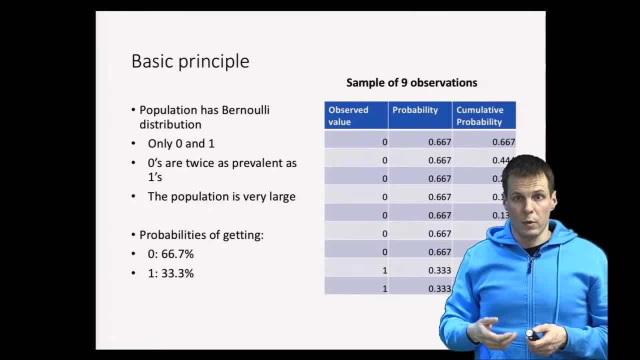 the population is not known, but we have to estimate what is the effect of age on menarche in the population and what is the probability of the population in the population. So it is an interesting thing to see and it would also be interesting to see that in this position. 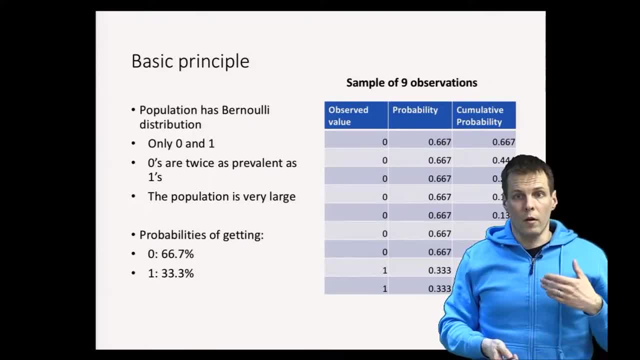 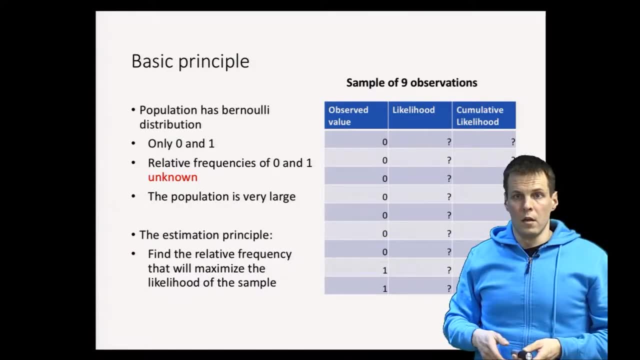 the base level, and so we don't talk about probabilities, we talk about likelihoods. So the idea of maximum likelihood estimation is that we try to find a population that has the maximum likelihood of having produced these values here. So we don't know what the mean is. 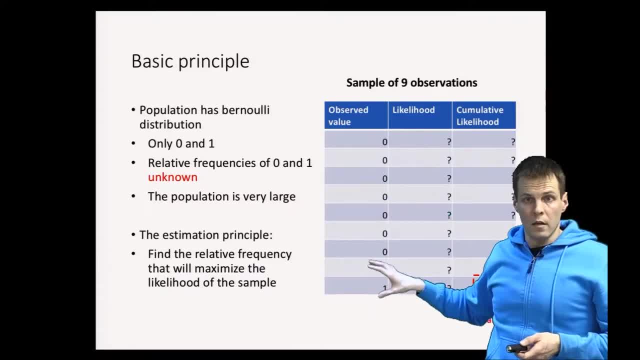 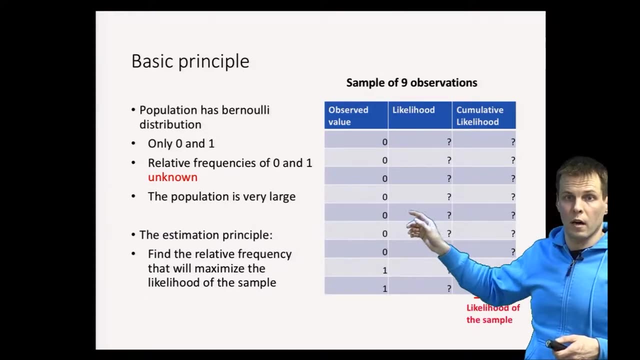 or what's the ratio of ones and zeros. we only know the data and we assume that the model exists for the population. Then we calculate, we have some guesses for this ratio and then we calculate likelihoods. we calculate the cumulative likelihood and we maximize the. 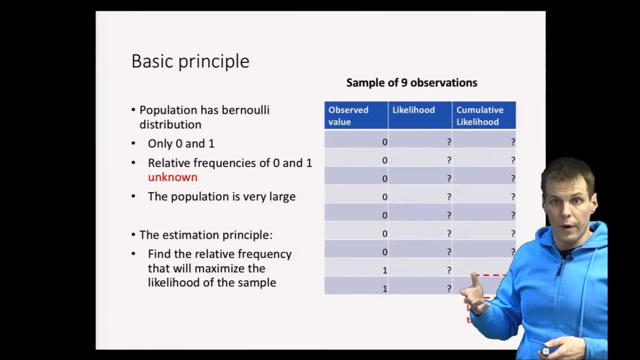 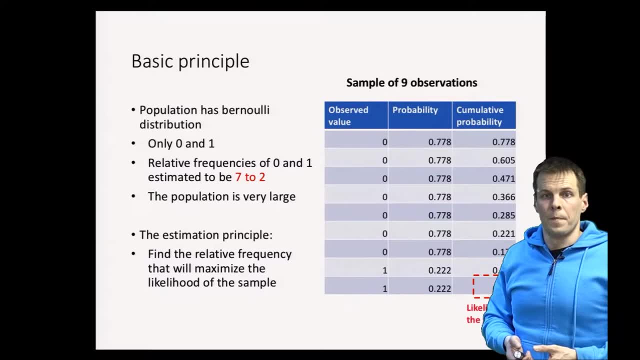 cumulative likelihood to find the maximum likelihood estimation by changing our model parameters. So, for example, we could guess that the ratio is 2 to 7, that gives us probabilities of 78% and 22% for zeros and ones. We calculate the cumulative probabilities and 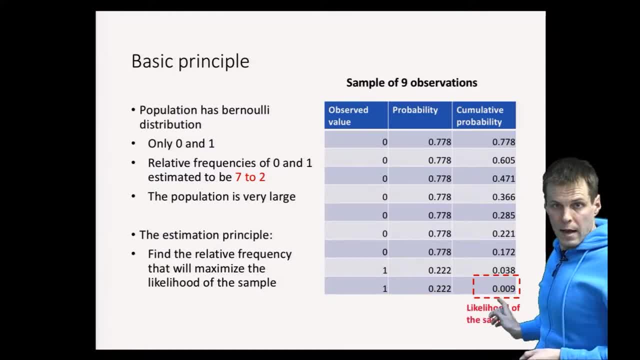 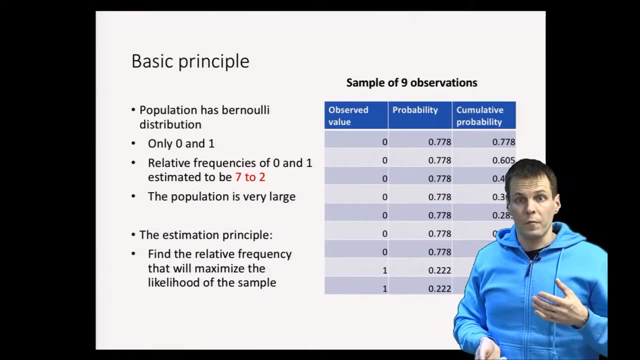 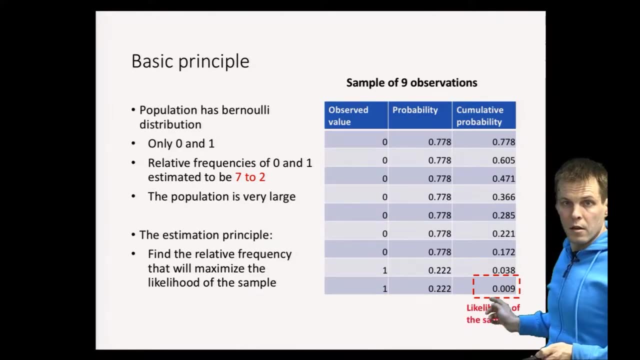 or we multiply everything together, and this is the likelihood of the sample, given our estimated population. The maximum likelihood estimate is simply found by changing our guess of the ratio of ones to zeros, so that this value here becomes as large as possible. This principle is applied. 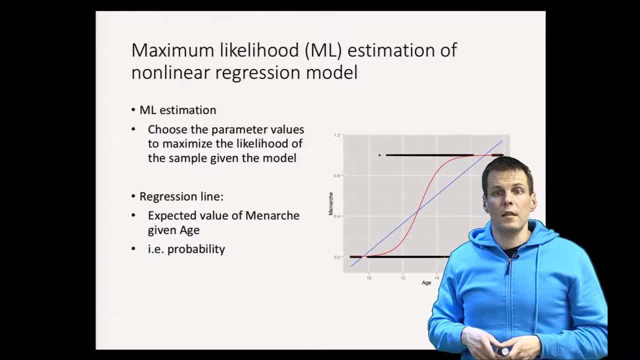 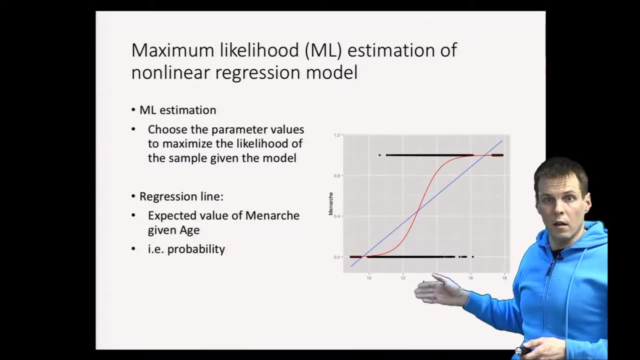 to the logistic regression analysis. The idea is that we calculate, using this logistic curve and this age here and the known ages and the known Menards- status of these girls. we calculate the individual likelihoods for the observations and then we use those individual likelihoods to find the best. 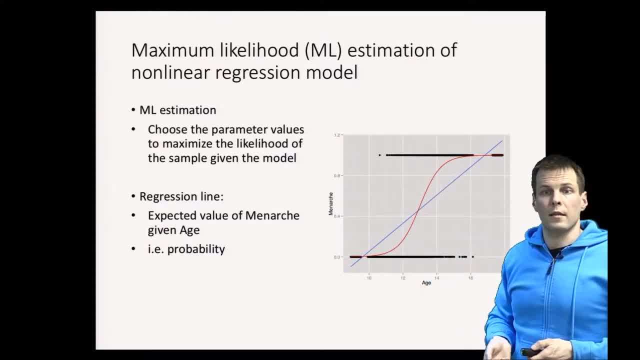 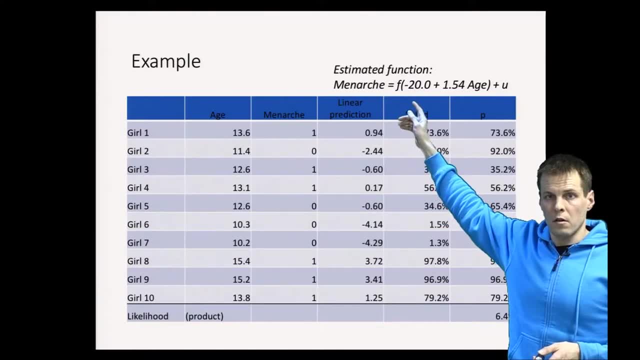 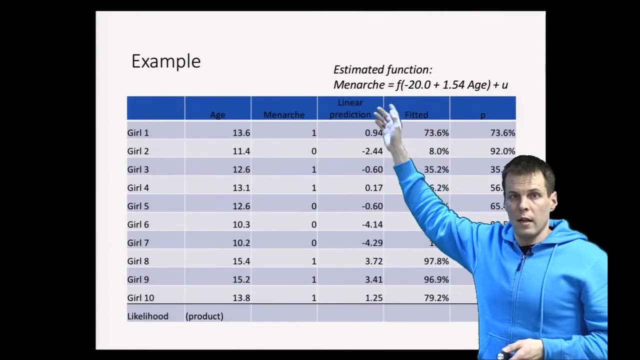 possible logistic curve for the data. How it works in practice is that we have some kind of guess. So we guess that Menards is a linear curve. we have some kind of guess that Menards is a linear function of age and an intercept transformed using the logistic function. So let's say that. 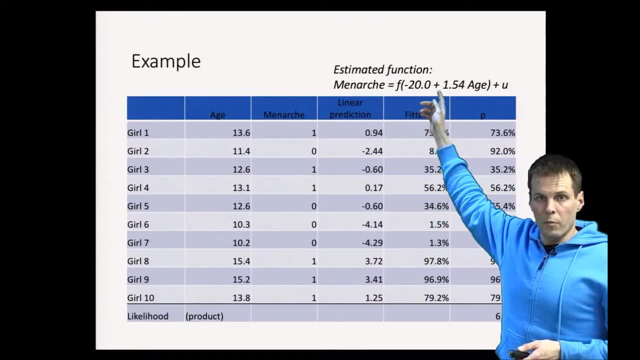 the intercept is minus 20 and the effect of age is 1.54, we apply logit function to the linear prediction and then we calculate That gives us the expected probabilities. Then we check how likely that particle observation is given the fitted probability. So for example, the first 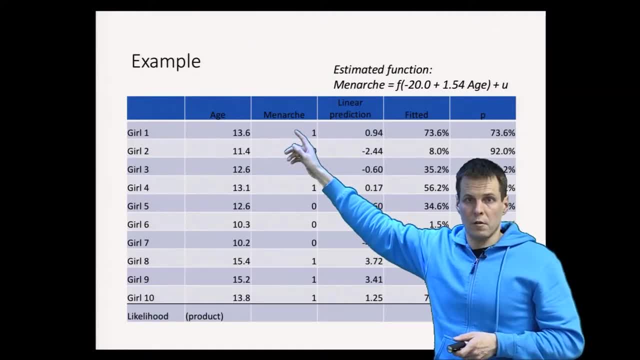 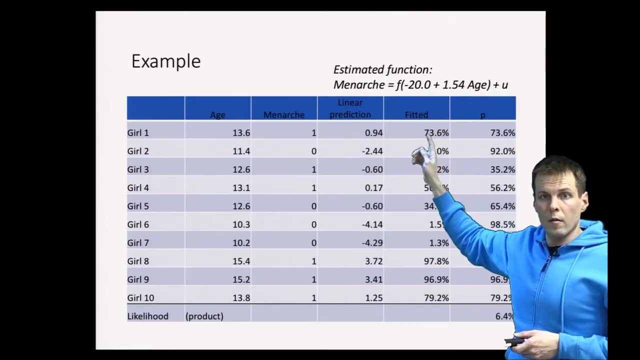 girl here is 13.6 years and she has had Menards. The linear prediction for that girl using this equation here is 0.94.. Then the fitted probability using the logistic function to this linear prediction is 73.6 percent. So if the probability is 73.6 percent and the girl has had Menards,